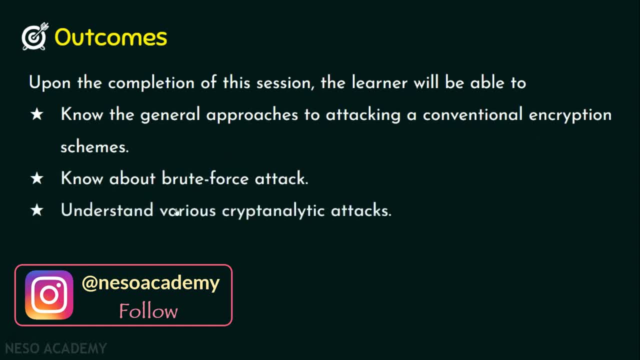 Outcome number 2, we will know about brute force attack. And outcome number 3, we will understand various cryptanalytic attacks. Before stepping into the various general approaches to attacking conventional encryption schemes, let's see a sample ciphertext. Here is the ciphertext: 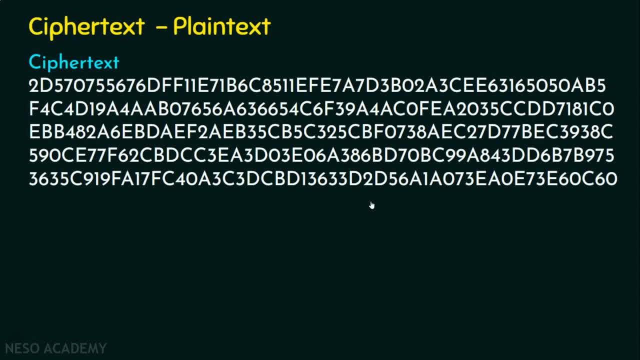 Can you figure out what is the plaintext for this equivalent ciphertext? I hope there is no way for you to know it, Because this is a scrambled text. this is the ciphertext, and I have not even provided what encryption algorithm that I use in order to generate this ciphertext. 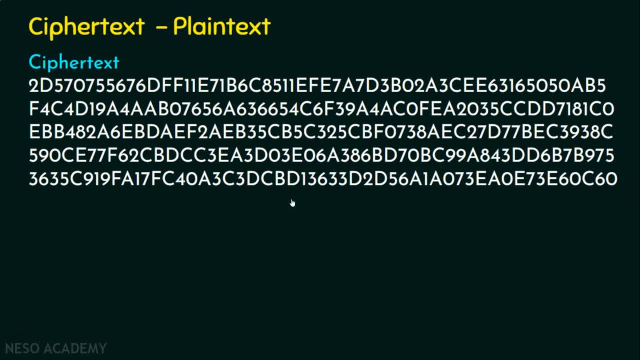 At the same time, key is obviously not going to be revealed, right? Even if I give the encryption algorithm, it's quite difficult for all to know what is the key that I have used in order to generate this ciphertext. Actually, the plaintext equivalent for this ciphertext is Hello World. 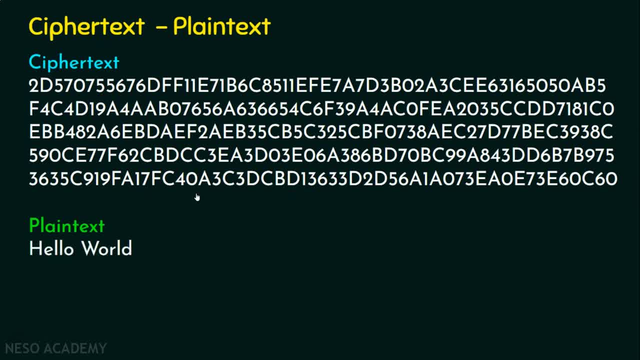 Trust me, guys, this is the plaintext and this is the ciphertext. for this plaintext, What algorithm did I use? The algorithm that I preferred for doing this task is RSA algorithm. It's a very popular algorithm. I am not going into the details of this algorithm. 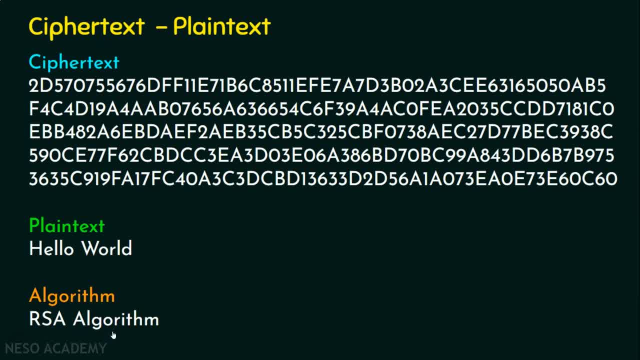 Anyway, we are going to see about this elaborately and we are going to solve many problems in the upcoming lectures, So for time being, we need to understand. if we have a ciphertext like this, it's very difficult to know what is the plaintext. 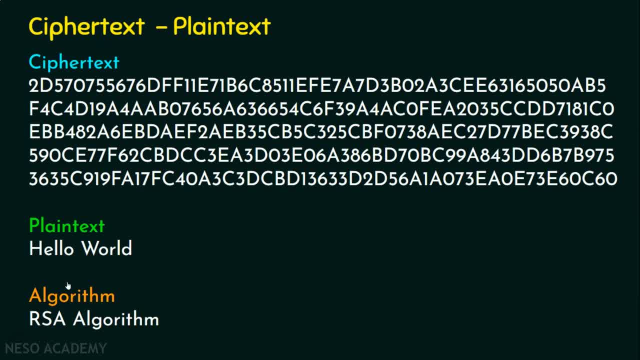 Because a ciphertext should be generated by an encryption algorithm, where this encryption algorithm should be the strongest one, which takes larger number of bit values in the key or a bigger key in order to generate the ciphertext. Only then it will be a secure ciphertext. Otherwise, attackers can easily attack the ciphertext and know what is the plaintext equivalent. 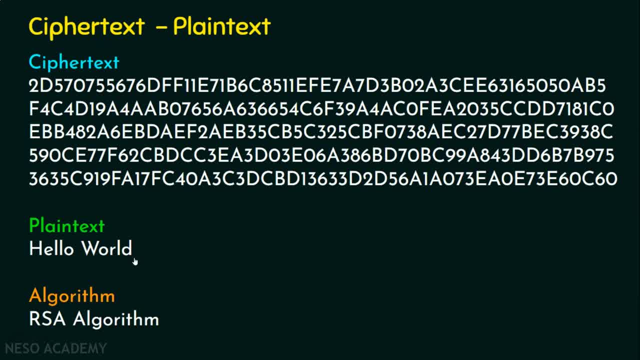 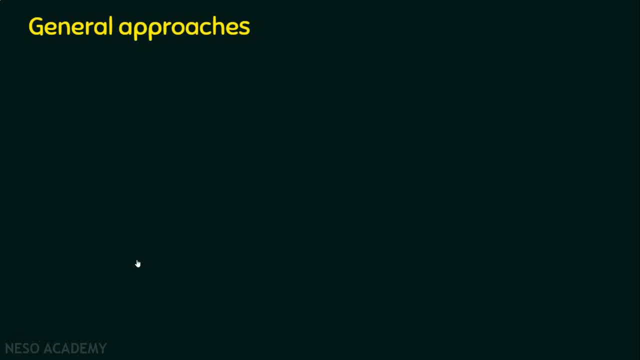 With this knowledge, we will step into the general approaches to attack the conventional encryption schemes, Since we have not seen the conventional or the classical encryption schemes. please make a note of this: All these conventional encryption schemes or classical encryption schemes are now obsolete. 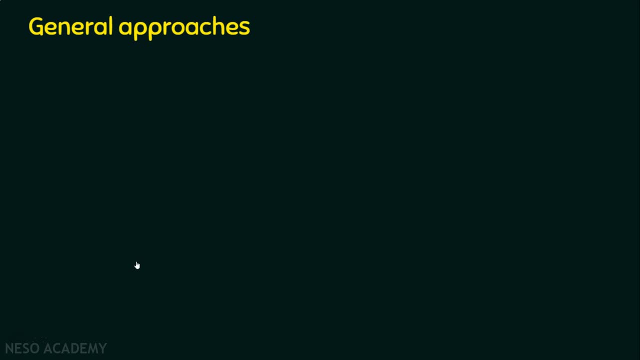 They are not used in today's world because it's very easy to hack and attack. Basically, there are two general approaches to attack A conventional encryption scheme. Number one is cryptanalysis, which we had already seen, And number two is brute force attack. 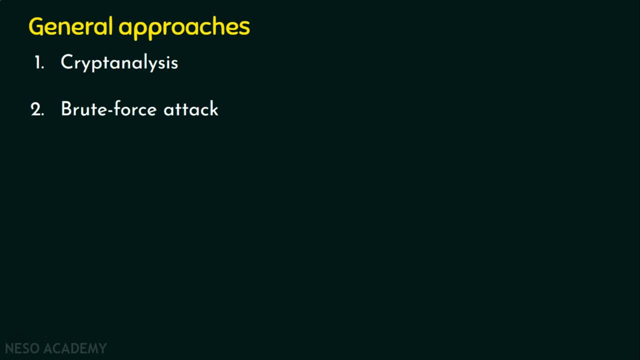 Cryptanalysis actually deals with how attackers or cryptanalysts will find the key based on some information available And coming to brute force attack, the attacker or the cryptanalyst will be trying all possible values in the key space. Suppose if there is a key space which contains a maximum of 50 key values. 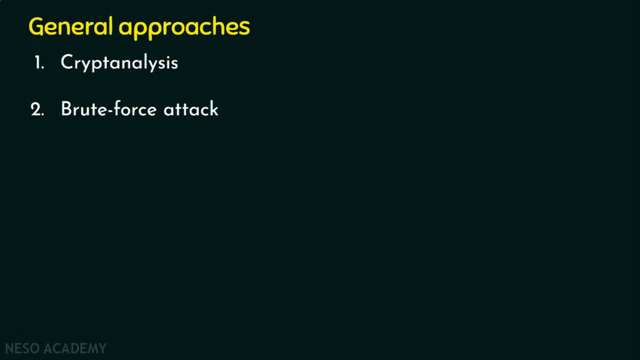 then the attacker will be attempting all 50 values in order to find the key. Anyway, we will be talking about that brute force attack in the next lecture. Let's first focus on cryptanalysis. What is this cryptanalysis? We have already seen this: attackers only will be doing cryptanalysis. 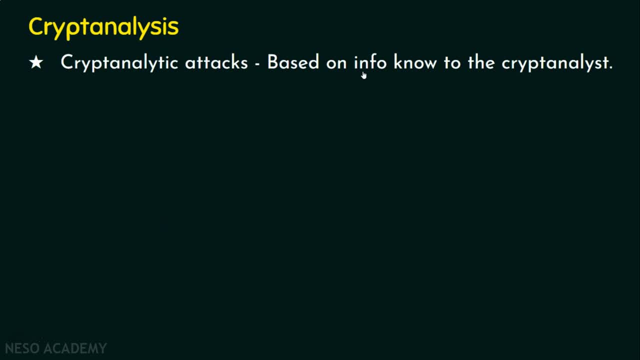 What is this? These cryptanalytic attacks are based on information known to the cryptanalyst, The person. the attacker is also called as a cryptanalyst because he is going to attack the system. right, He is going to find out what is the key. 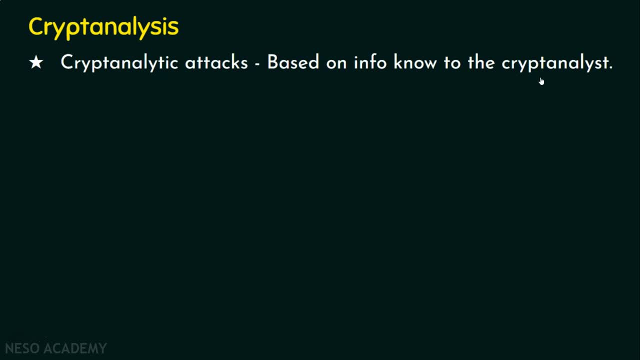 This cryptanalyst will be mainly focusing on finding the key which was used to generate the ciphertext. what he has received right. Definitely, ciphertext will be known to the cryptanalyst, but not encryption algorithm. But we assume that in this lecture series the cryptanalyst also knows about the encryption algorithm. 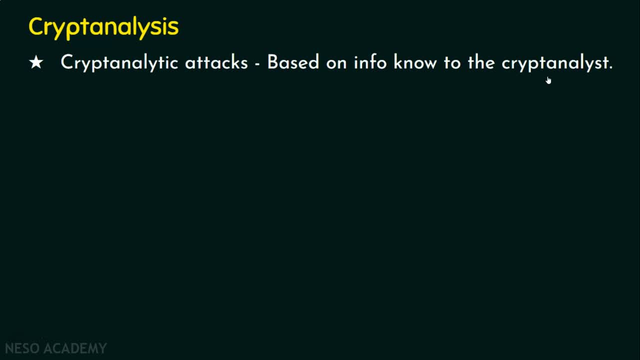 But anyway, key is the most secured one, which should be kept 100% secret. So from this we can understand that the cryptanalyst have some knowledge. What knowledge About the nature of the encryption algorithm? or some knowledge of plaintext ciphertext pairs? 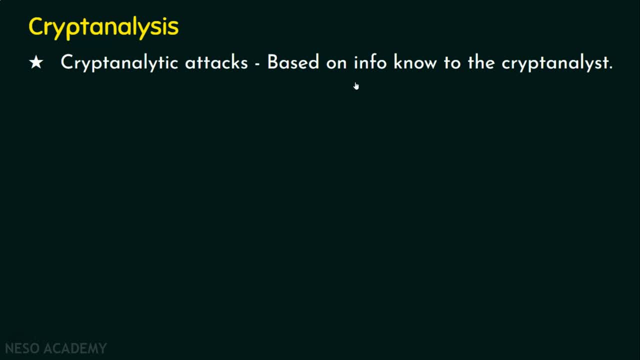 Basically, if the key is kept secret, then the cryptanalyst will be able to find the key. Basically, if the key is kept secret, then the cryptanalyst will be able to find the key. If the key space is a large key space, it will be very difficult to attack. 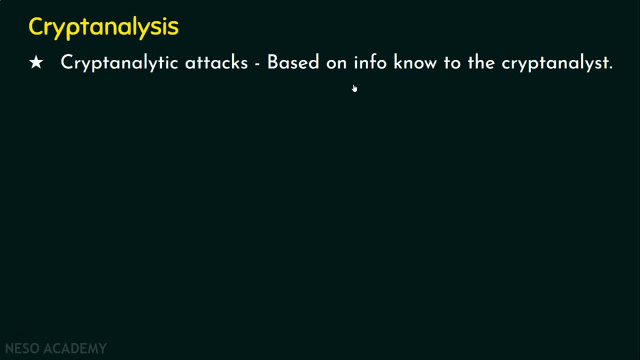 If the key space is small, then it will be easy to break, So we need to prefer the key space which is bigger as long as it could be. So this is basically about cryptanalytic attacks. So if the attacker receives only ciphertext and if he doesn't even know what is the 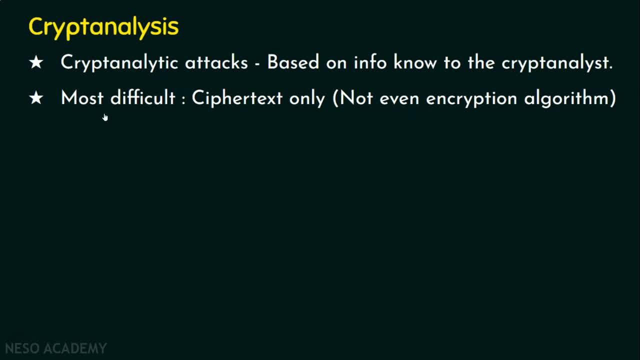 encryption that is used in order to generate the ciphertext. this will be the most difficult one, Because attacker has only the ciphertext. the cryptanalyst has only the ciphertext. He doesn't even know what encryption algorithm was used in order to generate the ciphertext. 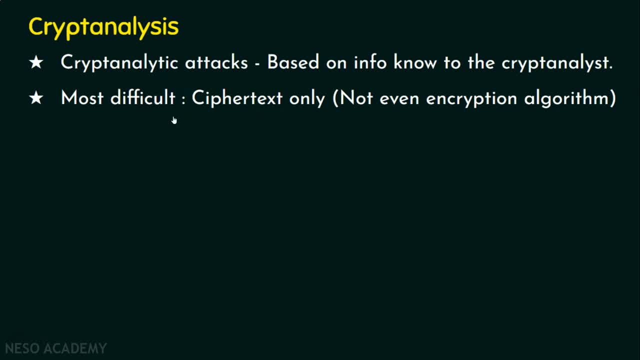 Obviously, key will not be known to the attacker, So this is the most difficult one as far as cryptanalyst is concerned. Please make a note of this type of attack: ciphertext only attack. Anyway, we are going to see that shortly. 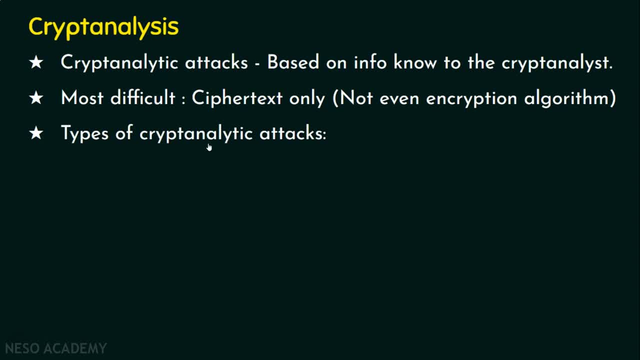 And coming to the third point, we have basically five types of cryptanalytic attacks: Number one, the ciphertext only attack. Number two: known plaintext attack. Number three: chosen plaintext attack. Number four: chosen ciphertext attack. And number five: chosen text attack. 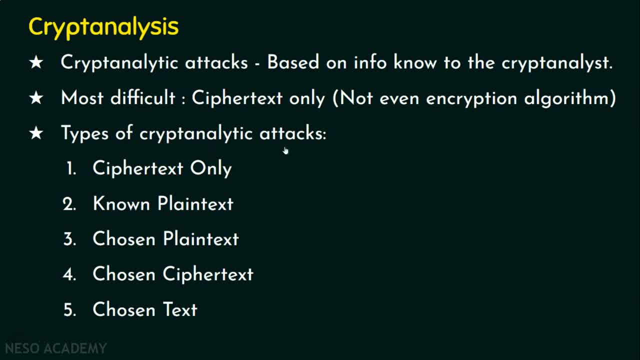 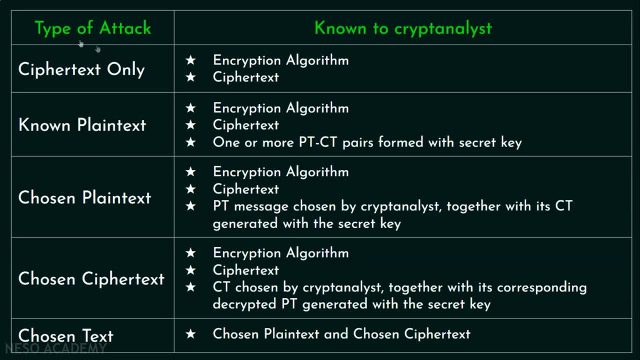 So basically, there are five types of cryptanalytic attack. Let's see one by one now. But anyway, I have consolidated the types of attack in a single slide. Here it is. We have the type of cryptanalytic attack in the first column and what information is. 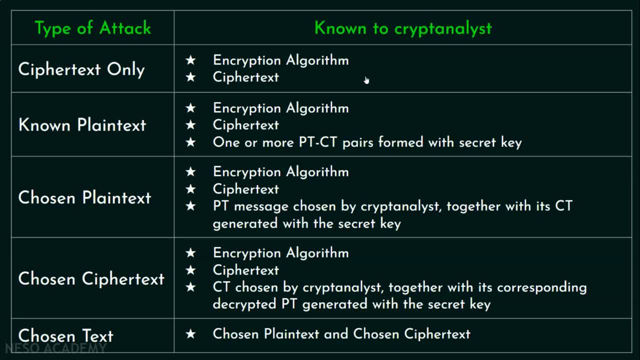 known to the cryptanalyst that is placed in the second column. Let's start with the first type: the ciphertext only attack. We have already seen this in the last slide, that this is the most difficult attack. Why? Because the attacker knows only the ciphertext. 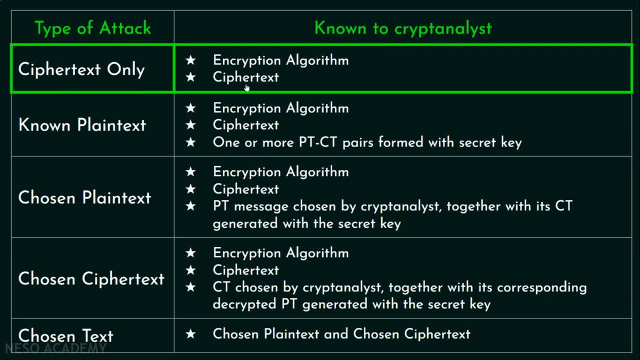 Can you see here, The attackers know, or the cryptanalyst know, only the ciphertext. As I already mentioned, we assume in this lecture series that the attacker knows the encryption algorithm also. So in all the types of attacks we can notice that encryption algorithm is known to the attacker or the cryptanalyst. 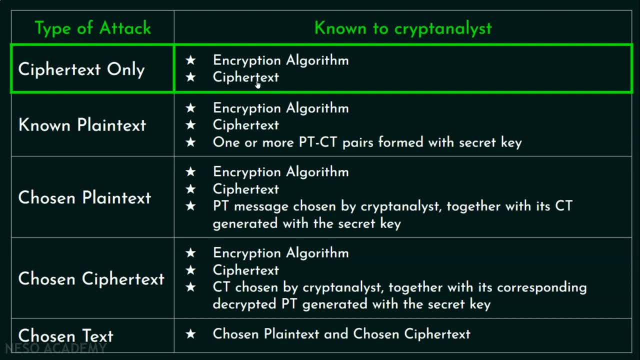 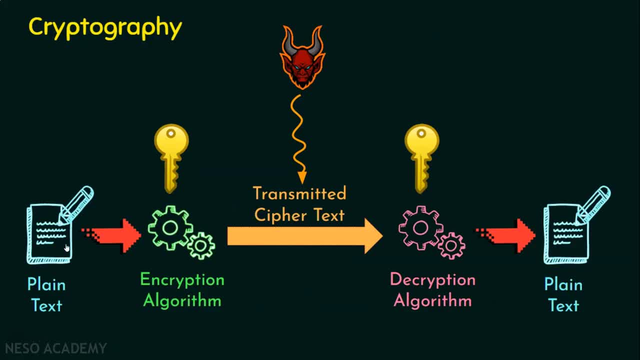 So encryption algorithm and ciphertext is also known to the cryptanalyst. You may be asking how ciphertext is known to the attacker. I will justify this. Just see this diagram. In this diagram we know the plaintext which is created by the sender. it is given to the encryption algorithm. 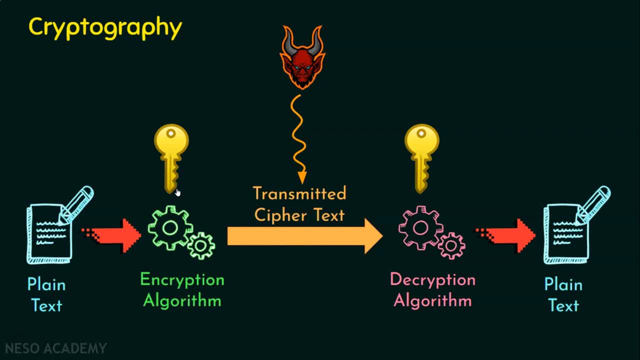 Whether it is a symmetric encryption or asymmetric encryption. just ignore about this now. Anyway, this encryption algorithm will be falling in one of the categories. Now this encryption algorithm will be producing this ciphertext and this ciphertext will be transmitted on the network. right? 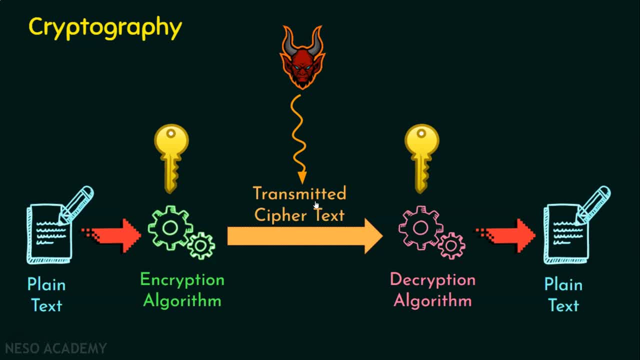 It may be on a network, it may be on the Internet, or it may be on the local area network, what so ever. Anyway, the ciphertext is going to flow through the network. Now, This is the transmitter ciphertext. When the ciphertext is transmitted, 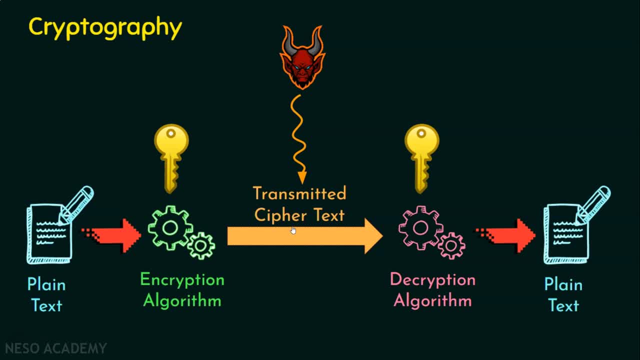 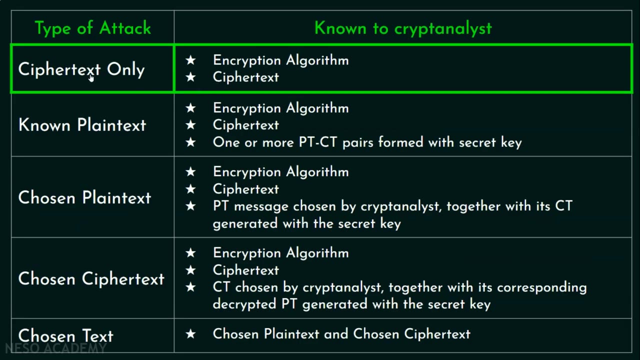 obviously attacker will have access to the ciphertext because ciphertexts are not confidential. We assume that the ciphertext will not be broken because we rely on a strong encryption algorithm with a strong key right. So ciphertext will be known to attackers also. So not only in ciphertext, only attack. in all the attacks ciphertext is known to cryptanalysts. 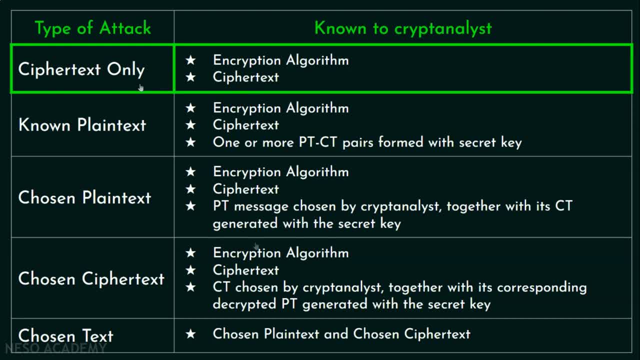 Can you see here: ciphertext is there in all the types of attacks. Now, talking about the first attack, the ciphertext only attack. we know attacker has only ciphertext and it is practically not possible to find out what is the plaintext or what is the key with just ciphertext, right? 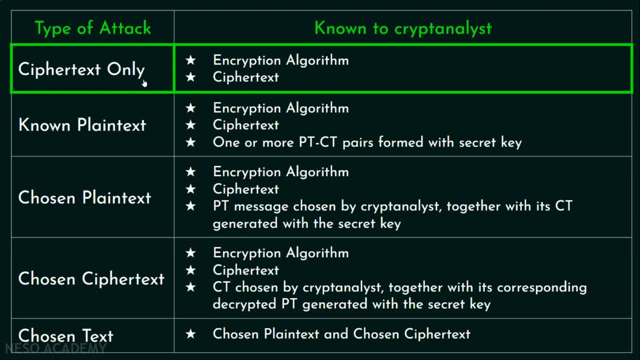 So this is about the first type of attack, the ciphertext only attack, which is the most difficult attack and this is the easiest way to defend. For us, it is the easiest way to defend and it is the most difficult one for the cryptanalyst. 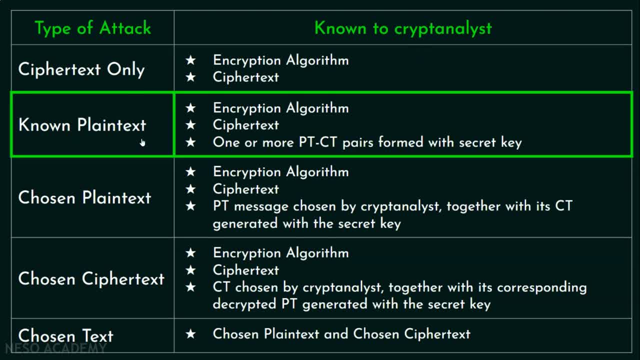 Coming to the second type of attack, the known plaintext attack. As already mentioned, we assume that the encryption algorithm and the ciphertext are known to the cryptanalyst. In addition to this, the name says that known plaintext, So the cryptanalyst knows certain plaintext. 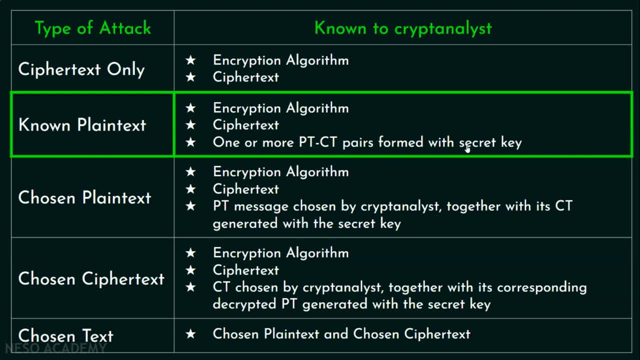 So one or more plaintext ciphertext pairs formed with the secret key. It's like the attacker or the cryptanalyst knows few plaintext ciphertext pairs. For example, for certain plaintext, what is the ciphertext? These details are known to the cryptanalyst and, based on this knowledge, 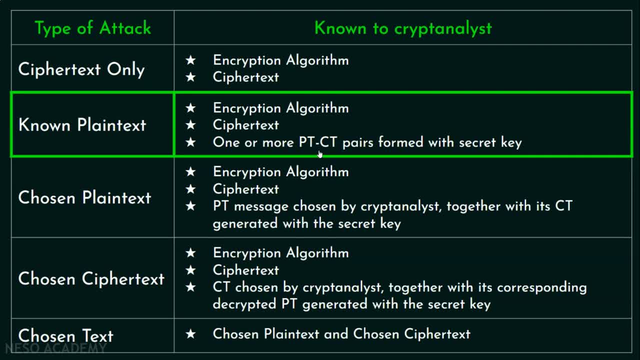 the attacker will be trying to find out what is the secret key. The attacker will be trying to know or find what is the key that is used to generate the ciphertext. This is known plaintext attack. Coming to the next type, which is the chosen plaintext attack, 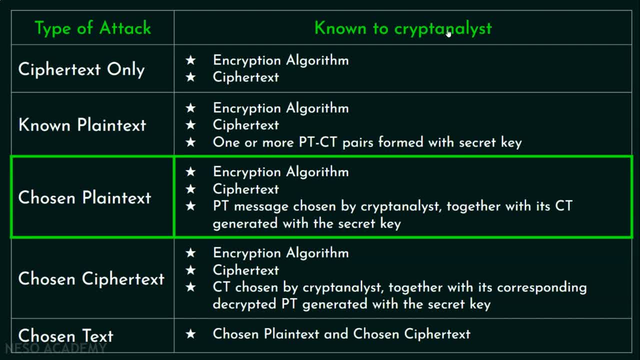 As usual, we know, the encryption algorithm and the ciphertext are known to the cryptanalyst. In addition to this, the plaintext message chosen by the cryptanalyst, together with its ciphertext, generated with the secret key. If this point is not clear for you to understand, let me explain it. 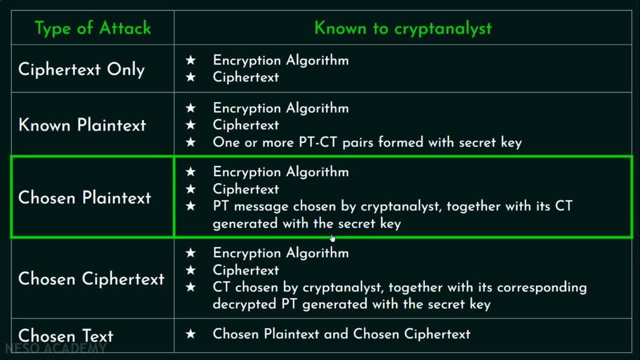 See, in the chosen plaintext attack, the attacker's intention will be getting the plaintext from the ciphertext, because ciphertext is already known to him. So now the attacker's intention, or the cryptanalyst's intention, will be getting the plaintext from the ciphertext. 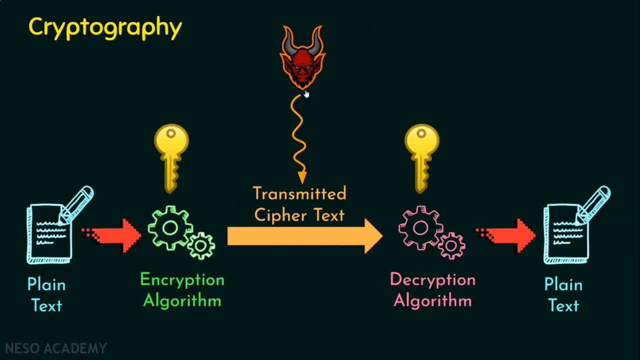 Let's see the diagram. Let's say he is involving in chosen plaintext attack. The attacker has the ciphertext right. So, without knowing the key, this attacker or cryptanalyst will be trying to get the plaintext from this ciphertext. For example, let's assume this attacker is given some temporary access to the encryption algorithm. 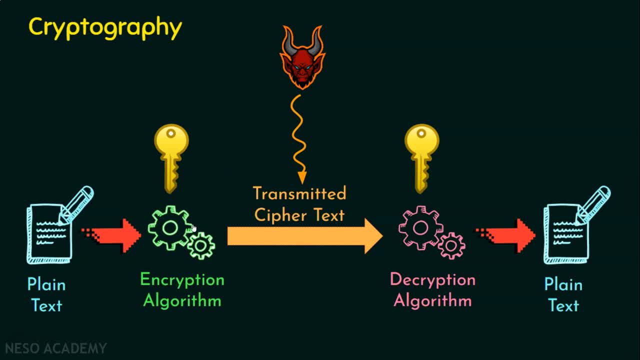 Now, in this case, he will try to feed certain plaintext and get the ciphertext. Now he has some knowledge about the plaintext-cyphertext pairs, So his intention will be getting the plaintext from the ciphertext, And not only this, let's say the analyst, the cryptanalyst to be precise. 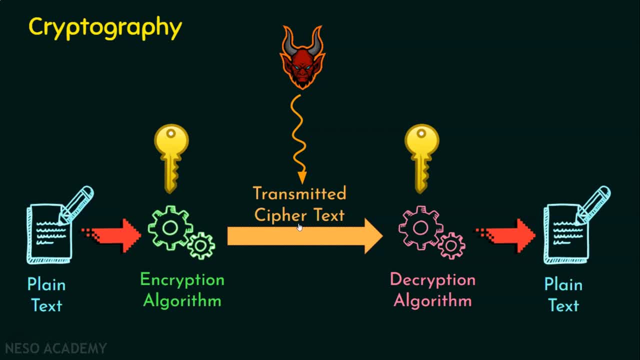 he is able to send or he is able to insert a message into the system And then he gets the ciphertext for the plaintext he has inserted into the system. So now he got some information about plaintext-cyphertext. He can guess it right. 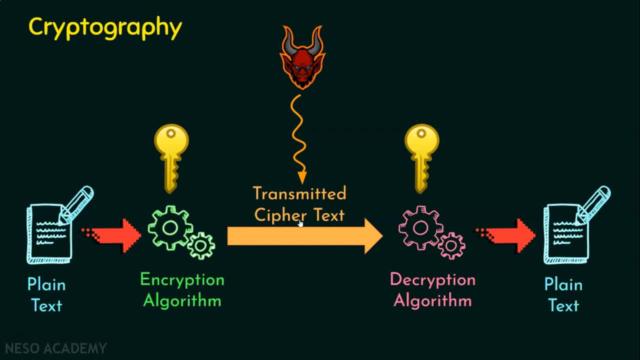 Based on this knowledge, he will try to break the ciphertext and find the key, The access. what the attacker gets in this example is just a temporary access And we assume that the attacker is granted the temporary access. So this is what the chosen plaintext is. 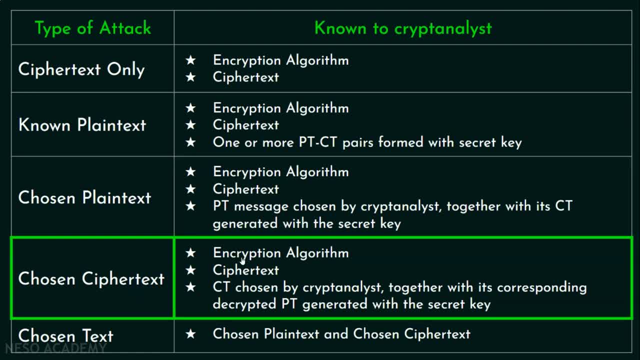 So, coming to the next type, which is the chosen ciphertext attack, We know the encryption algorithm and ciphertext are known to the cryptanalyst, But here the ciphertext chosen by the cryptanalyst- in the previous case, the plaintext message- was chosen by the cryptanalyst. 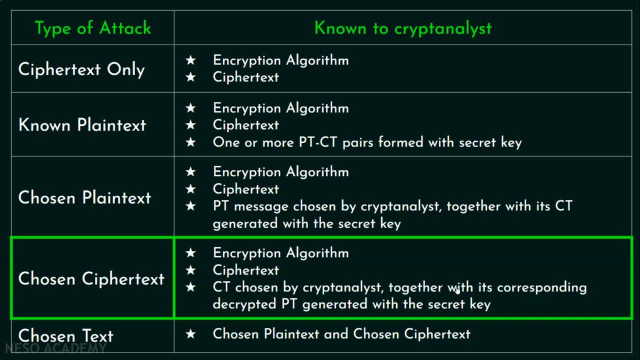 Now the ciphertext chosen by the cryptanalyst, together with its corresponding decrypted plaintext. it means the ciphertext was decrypted and we get the plaintext back. So ciphertext chosen by the cryptanalyst, together with its corresponding decrypted plaintext. it's not simple plaintext, it's decrypted plaintext. 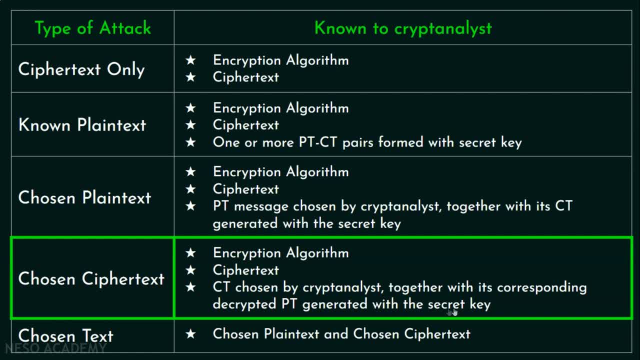 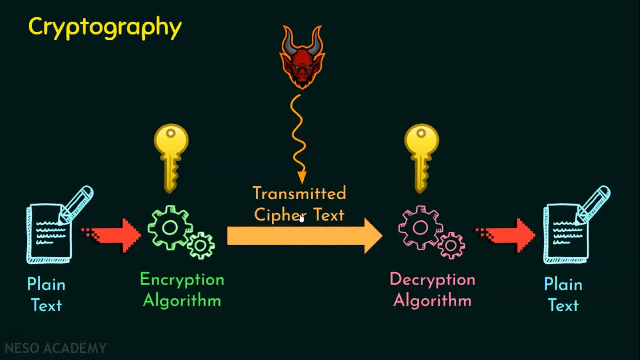 After decryption, we get the plaintext back, generated with the secret key. To understand this point, just imagine we get temporary access to the decryption algorithm. Let's see the diagram. In this diagram. in the previous case, the encryption algorithm access was given to the attacker. 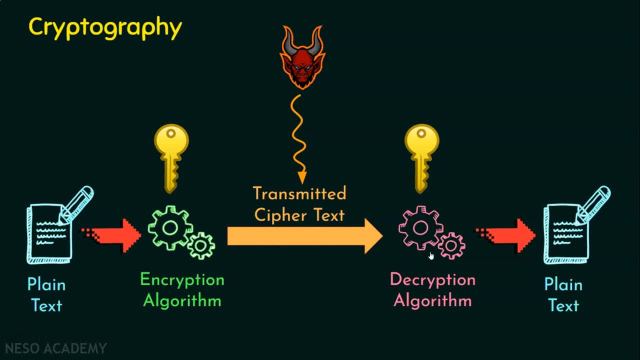 Now let's assume this attacker is able to get some access to the decryption algorithm In order to decrypt the ciphertext. he has the ciphertext right, So he gives the ciphertext to the decryption algorithm and gets the plaintext. So he will now have certain ciphertext and decrypted plaintext. 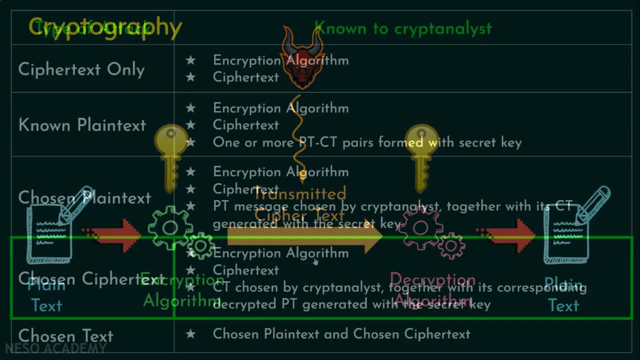 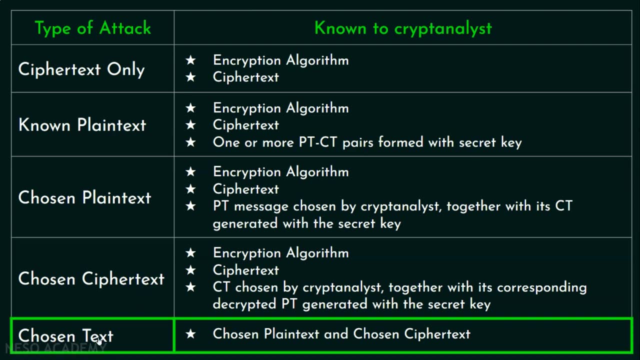 With this approach and knowledge, the attacker will try to find the key. So this is all about the chosen ciphertext attack And coming to the last type of cryptanalytic attack, it is chosen text attack. It is the combo of chosen plaintext. 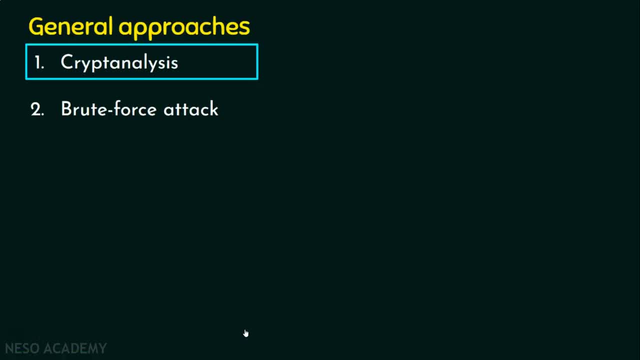 and chosen ciphertext attack. We are done with the first general approach of attacking the conventional cryptosystem, which is the cryptanalytic attack. We will see the brute force attack in the next lecture, And that's it, guys. I hope now you know the general approaches. 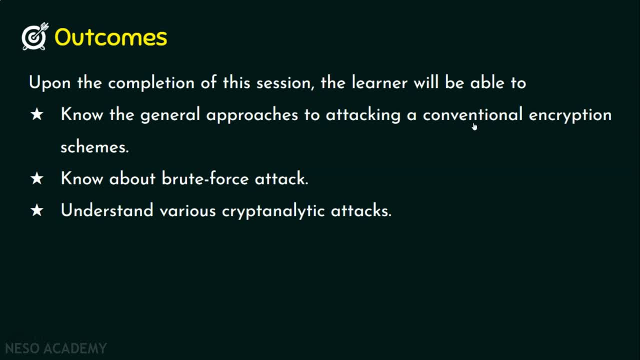 the cryptanalytic attack and the brute force attack to attacking a conventional encryption scheme. We also have seen brute force attack in brief, and we also have understood the various cryptanalytic attacks. I hope you guys enjoyed today's lecture and thank you for watching. 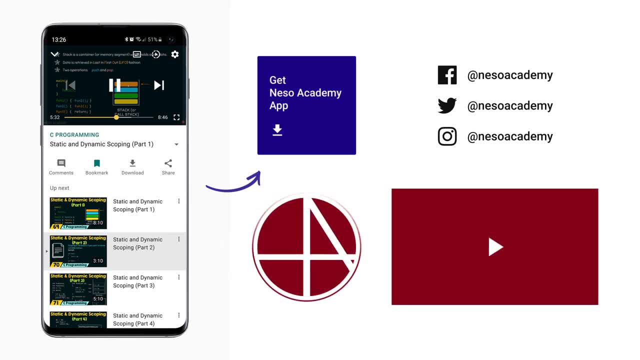 I'll see you guys in the next lecture. Bye. 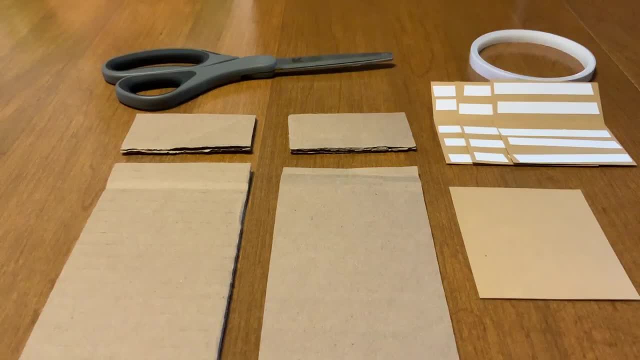 Solo board gaming night here and I just wanted to show you how I make my custom inserts. Some people might be a little bit intimidated, thinking that it may be too difficult, but literally with the pencil, a roller, scissors, double-edged tape, some regular old cardboard paper and some craft. 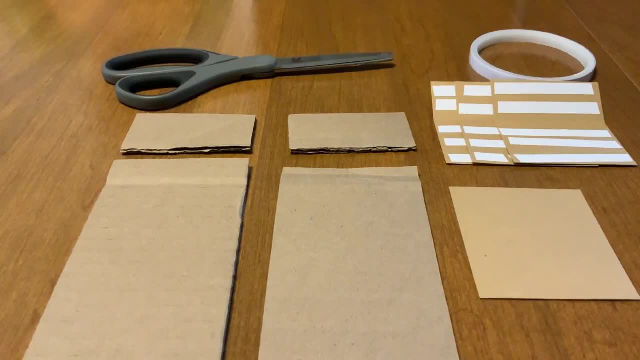 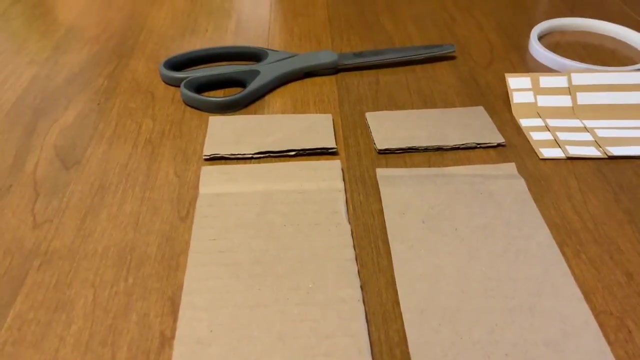 paper. you would be amazed how easy, fast and very effective it would be to make an insert to help store your favorite games, like Journeys in Middle Earth, for example. So I'm going to go ahead. I already went ahead and cut out the pieces of cardboard. Now this is just an example. I didn't. 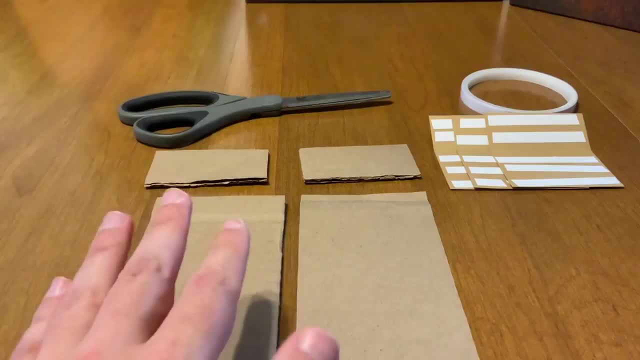 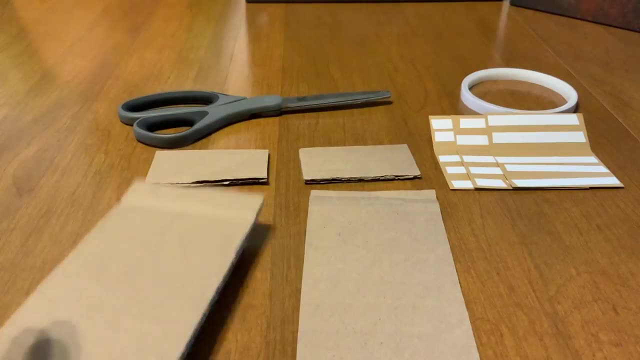 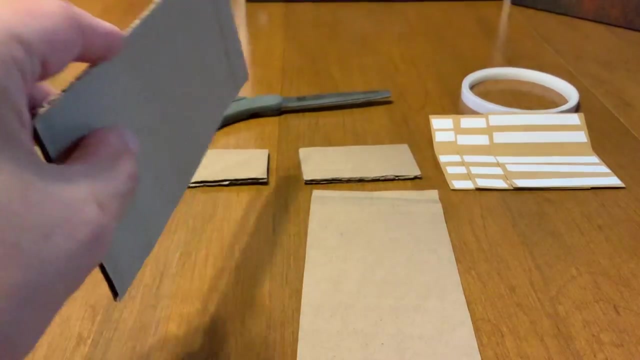 go ahead and make one exactly the size. I just wanted to show you through example how easy it is to do, So I just went ahead and cut it. Just make sure that you measure the inside of the box length and width and that you cut it up for an appropriate size and always also like insert it.